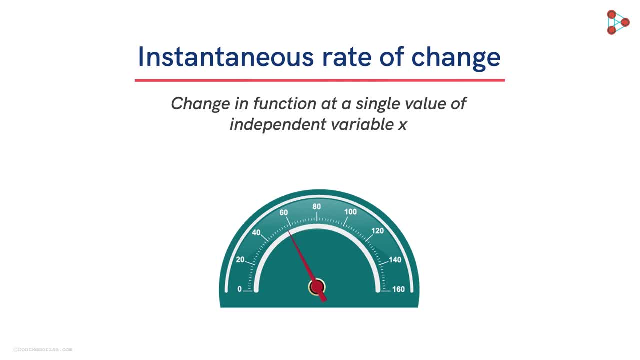 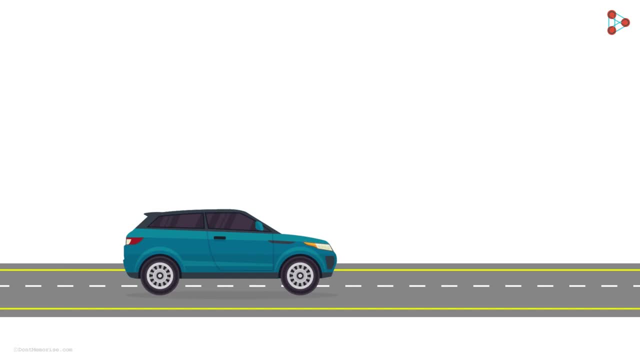 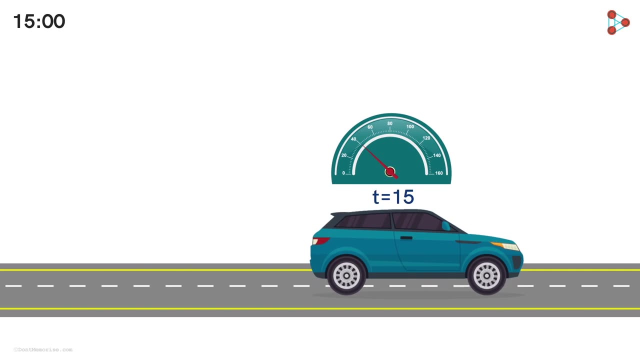 The reading in a speedometer tells you how fast you're changing your position roughly at that particular instant of time. when you look at it, Imagine you start at a time t equal to zero And after 15 minutes into the journey the speedometer reads 40 miles per hour. 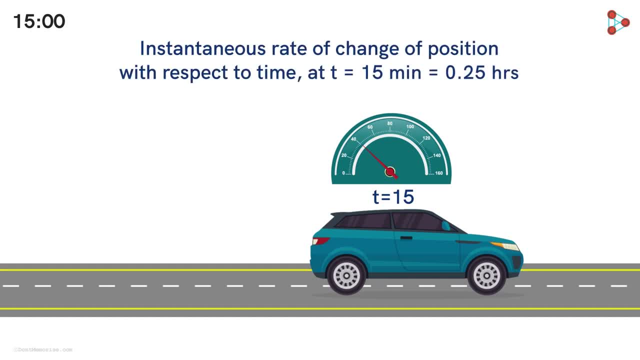 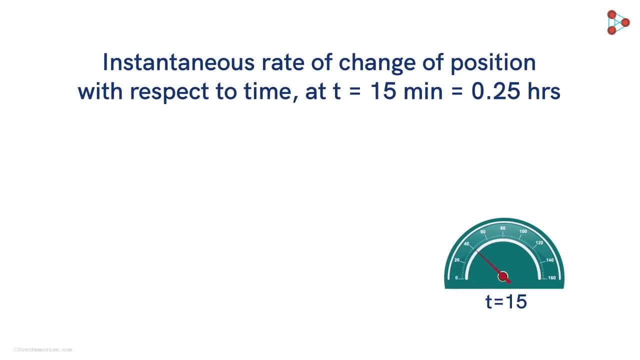 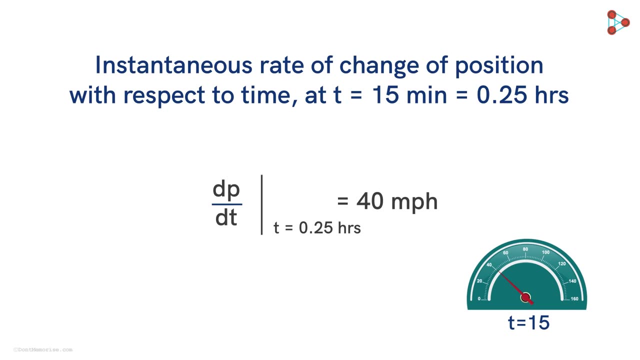 Now that's your instantaneous rate of change of position with respect to time, at t equal to 15 minutes or 0.25 hours. It's written as dp dt, followed by a vertical line and down in the subscript t equal to 0.25 hours. 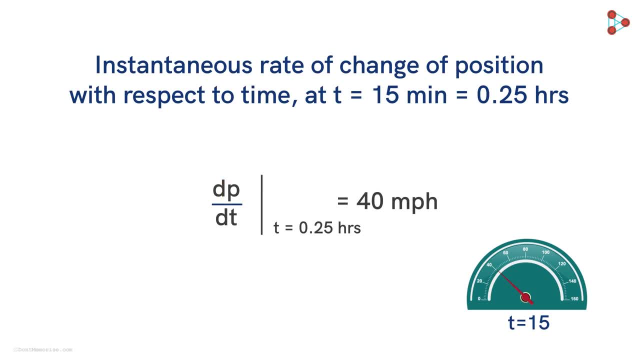 where p stands for the position And that's the derivative of the position with respect to time at this particular instant of time. Derivative as rate of change of quantity has many practical applications where we are looking for how fast one quantity is changing with respect to another quantity. 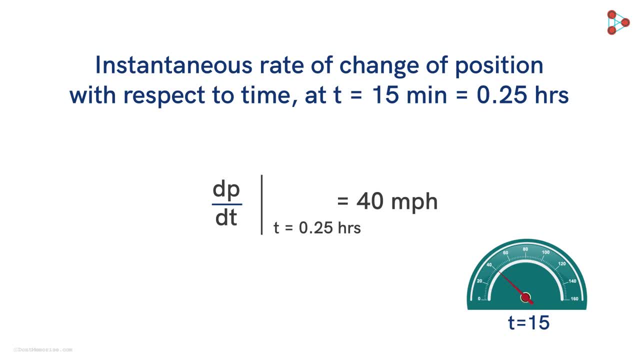 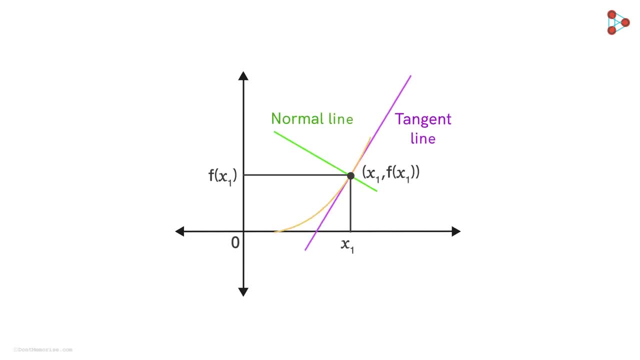 And we will start our study on it starting from the next video. Another application of derivative is to find the equation of tangents and normals at a point on a curve. Like I mentioned in the beginning, the geometrical interpretation of derivative at a point. 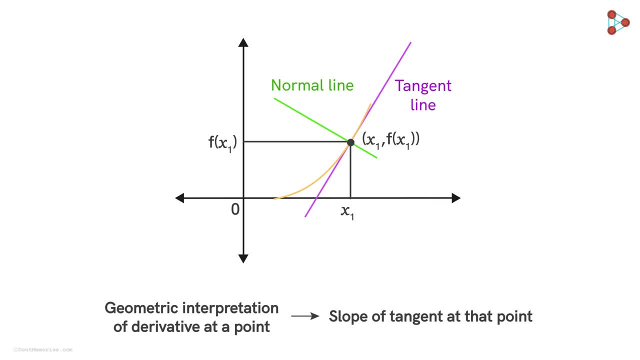 is the slope of a tangent at that point, usually denoted by a small letter m. If we know the slope of any straight line as well as the coordinates of any one point on it, then the equation of that line can be found by point-slope form. 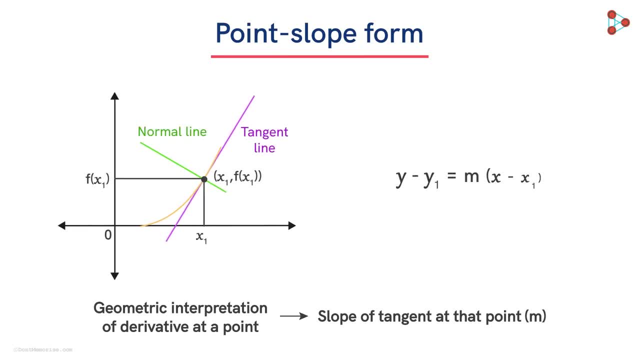 I am talking about this popular form, y minus y1, equal to m times x minus x1.. Here, x1 comma y1 are the coordinates whose values are known to us, and m is the slope of the line. In our case, the derivative is the slope. 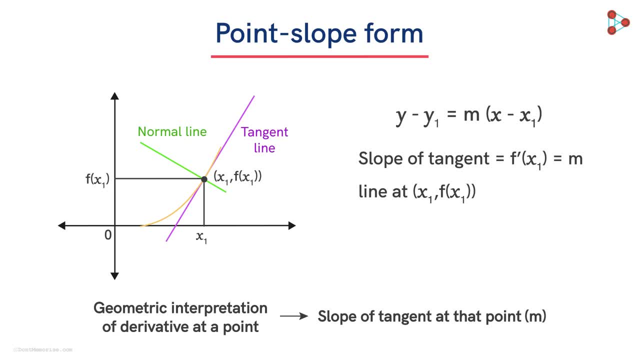 and the known coordinates will be x1 comma f of x1, the point where the tangent touches the curve. The equation of the tangent at x1 will then be y minus f of x1, equal to f prime of x1 times x minus x1. 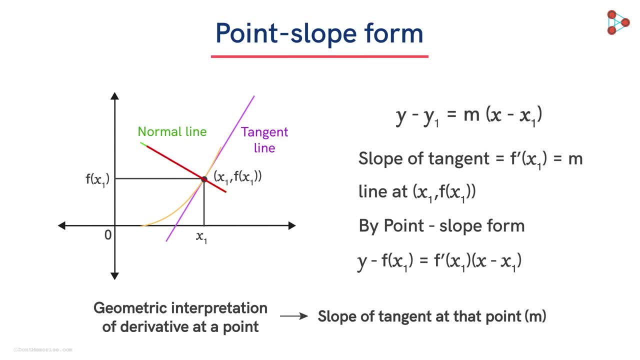 In a similar way, we can find an equation of the normal line which is perpendicular to this tangent at the point of tangency. More on that in the upcoming videos. Now, once we know how to find the equation of a tangent line using derivatives,